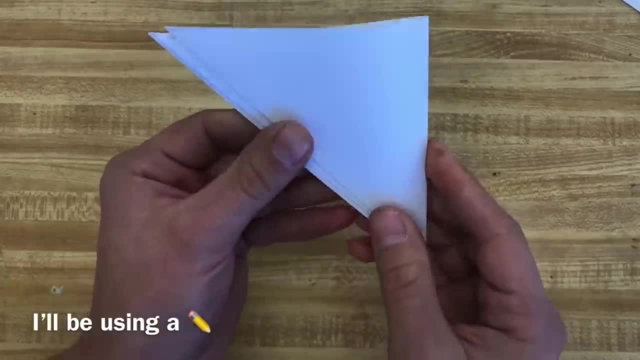 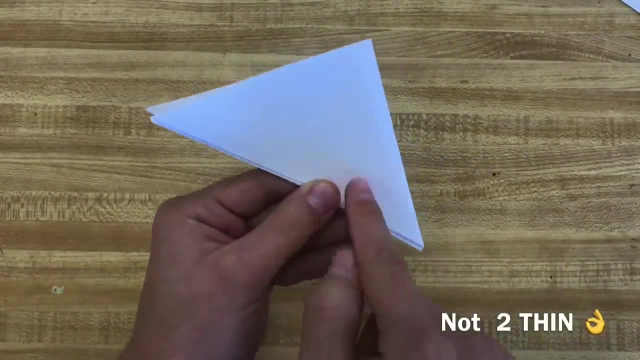 different parts of here. Just make sure that you do leave some of these folded edges. The edges that are folded have to still have something left. If you cut up all of these or make them really, really thin on here, it's going to open and rip apart. So I'm going to just do a basic 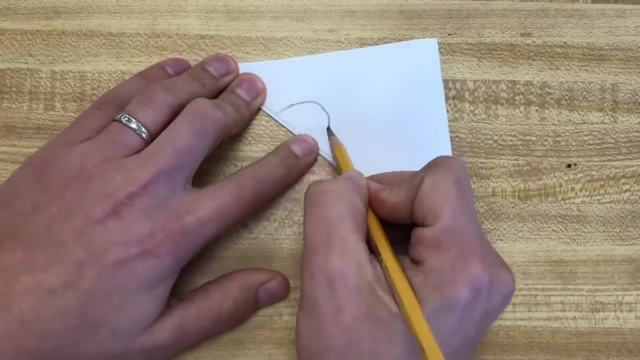 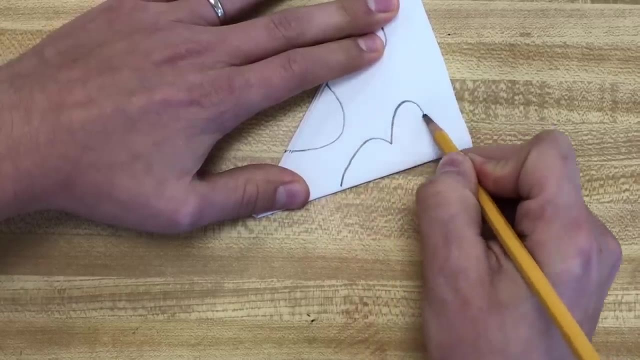 little design. So I'm going to do one, two, and then let's give it a little bump over here. One, two, a little lump on there, And then you can cut that out, And then you can cut that out, And then. 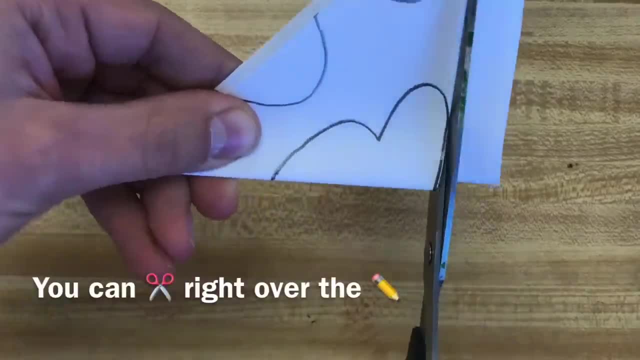 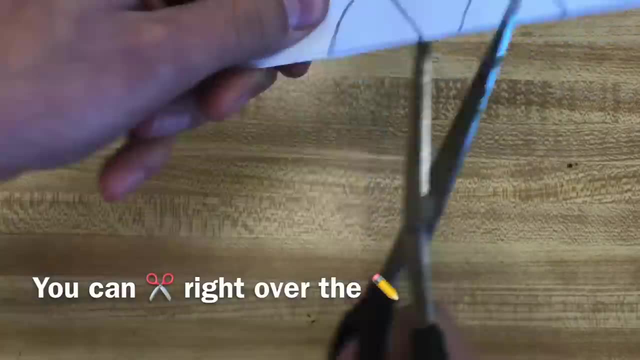 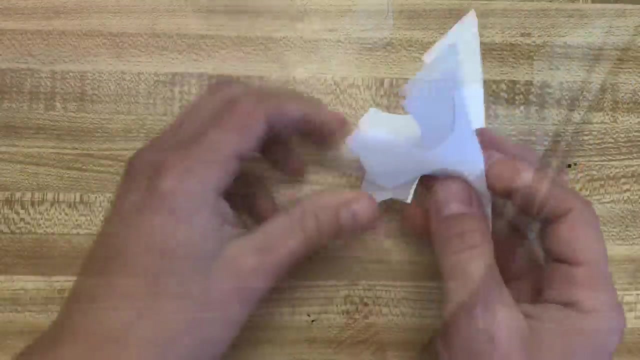 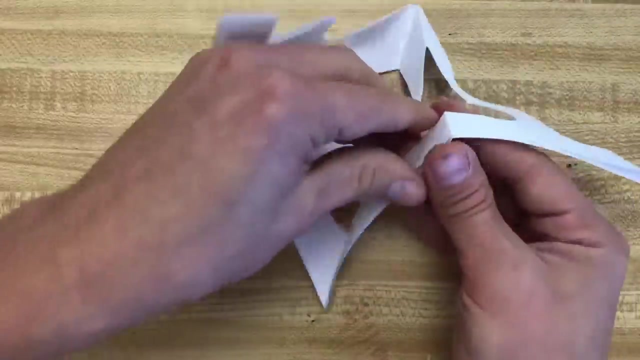 you can cut those out. So I'll go through that real quick. All right, let's see how this one looks now. So it's got those shapes out of there. So then when you open it up, you can see it gets a little bit bigger and a little bit bigger. 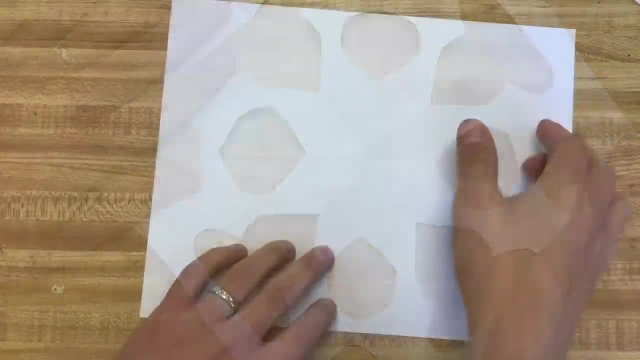 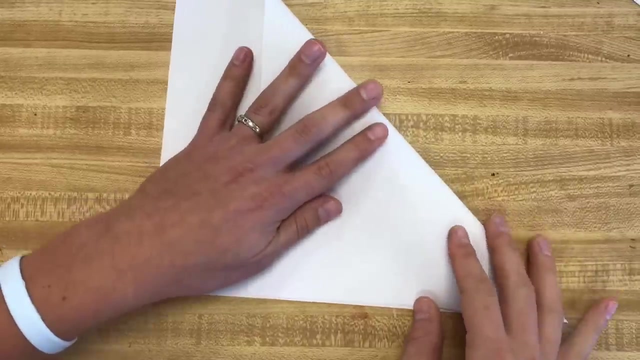 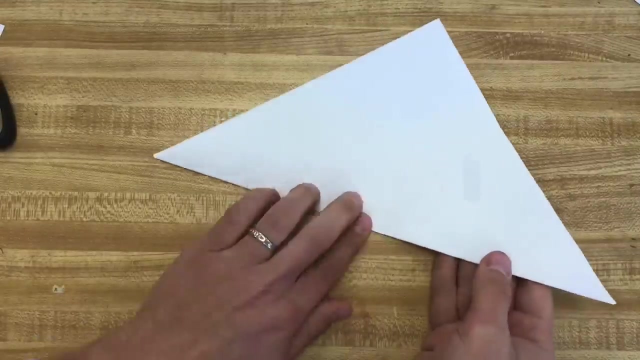 Oh, I like that. That looks really really cool. I'm going to go through really fast because you guys paid attention in the first part, So I'm going to fold it again right across, And I got my little triangle again This time I'm going to do. 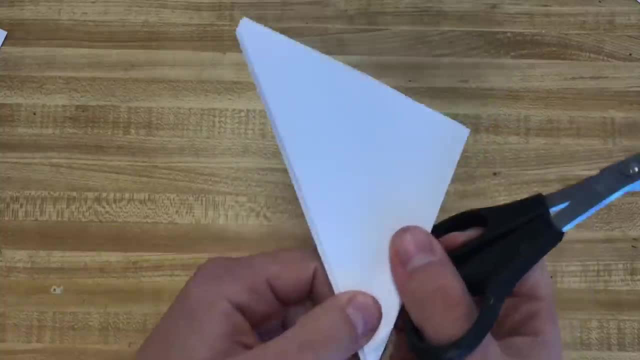 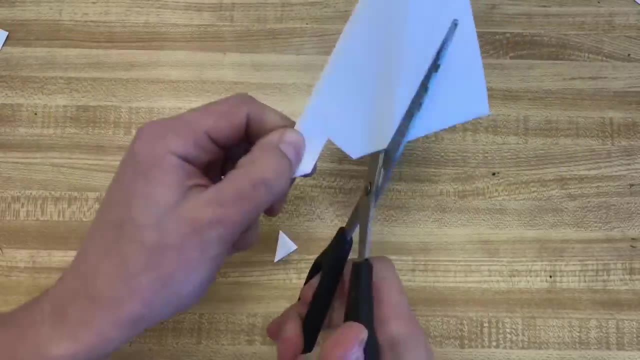 like I said, more of a freestyle version. So I'm just going to go all the way around the edges and do little itty bitty triangles. So I'm going to go in and out, in and out And go all the way around the outside, still leaving. you can see how it. 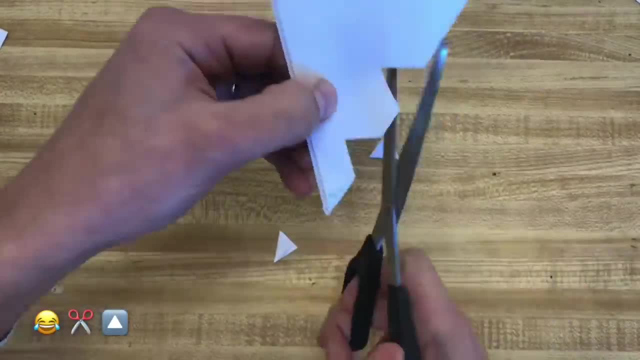 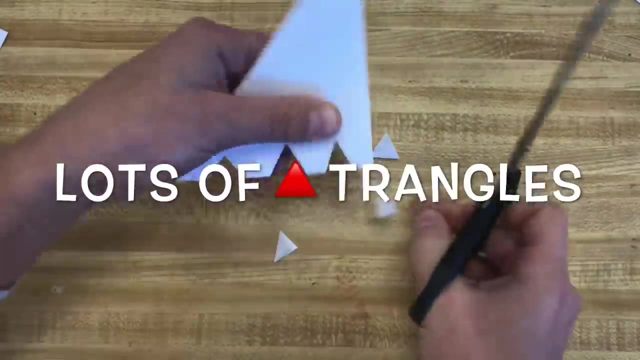 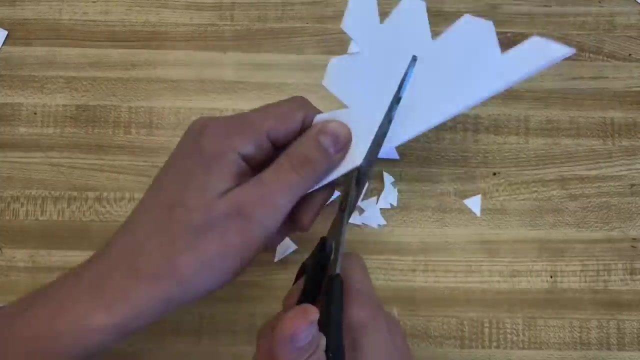 sticks in there, sometimes still leaving a little bit of that folded edge on here, Not going so close that it's going to be really flimsy. So I still want it to be strong, So let's go through that real quick. So this is probably what I would say the most popular. 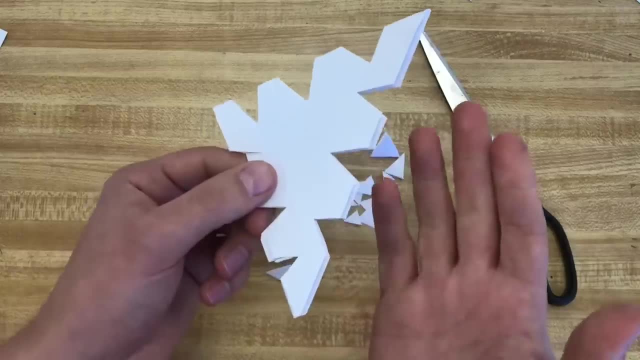 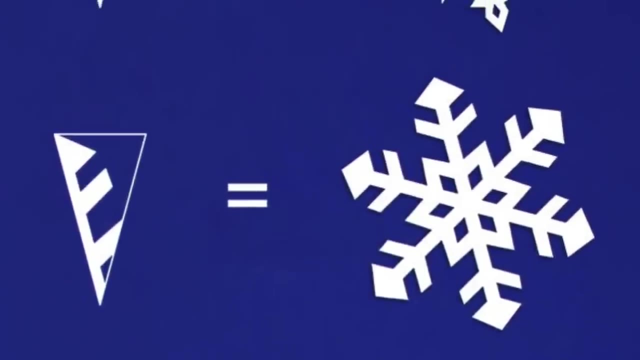 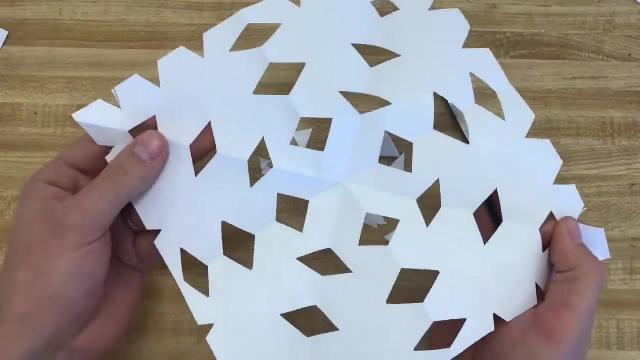 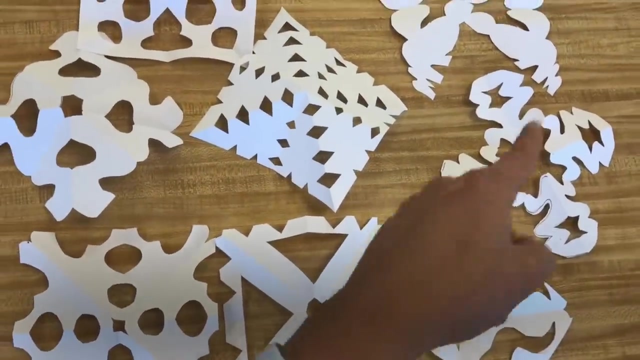 one You can see different designs. There's actually really super cool designs online that you can just. it gives you kind of a little stencil that you can draw different things and then cut them out. Well, this will look Bam, Look at that Awesome. I will put a link also in the bio for some of these more complicated.